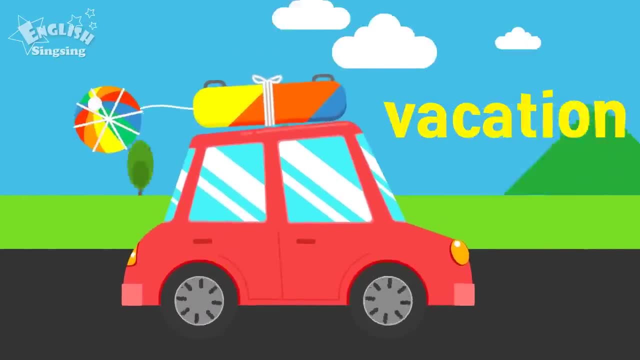 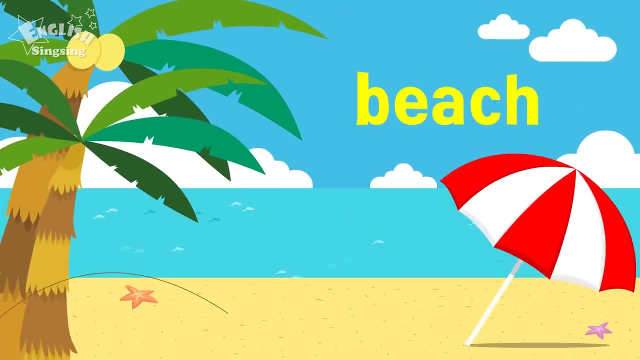 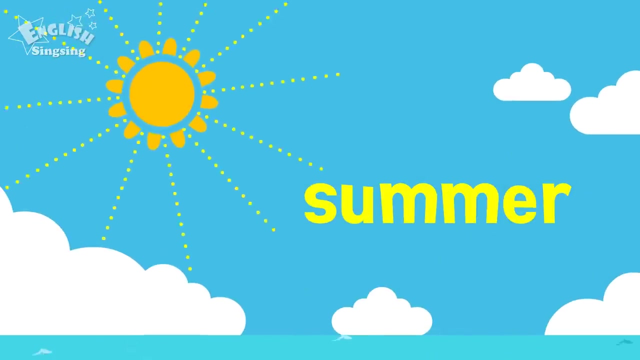 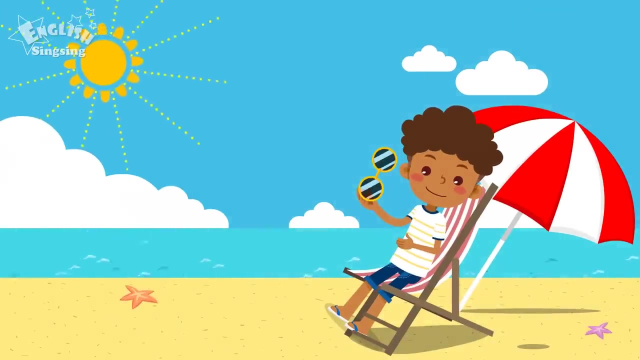 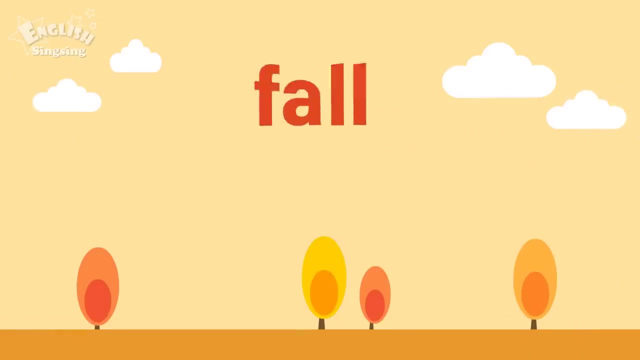 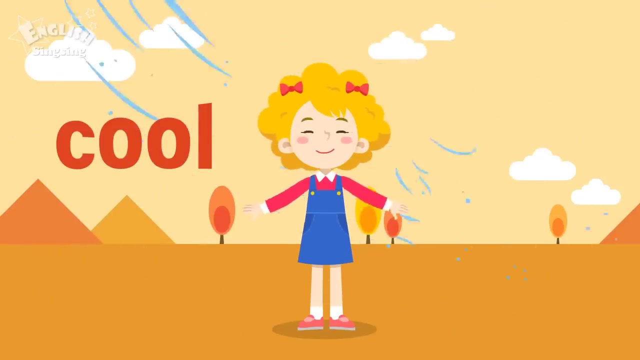 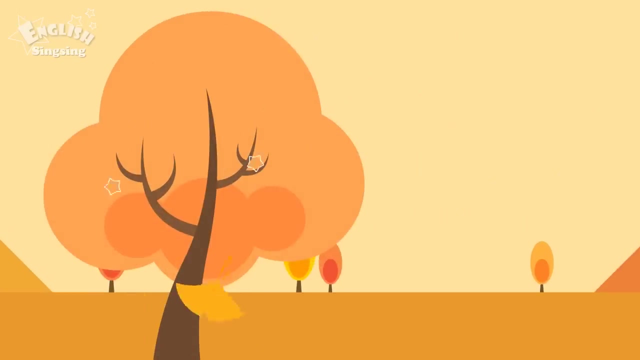 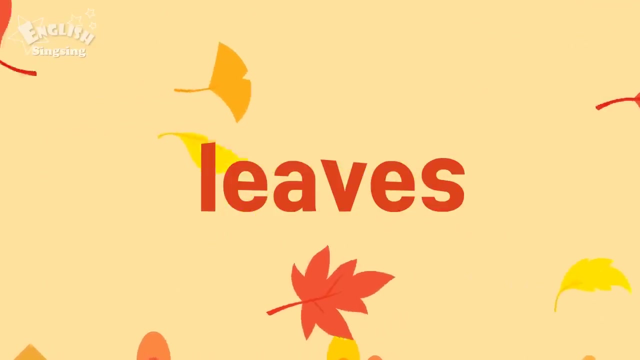 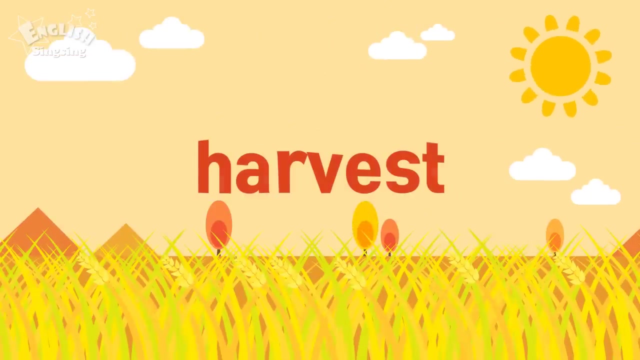 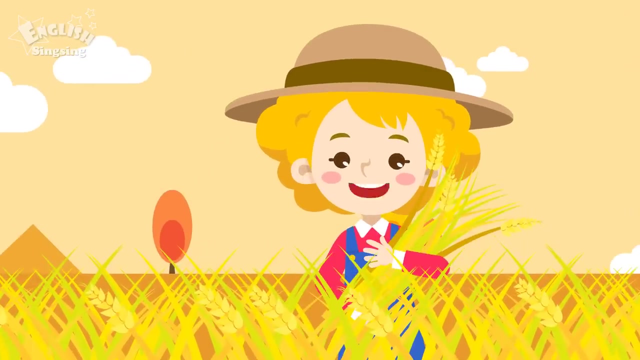 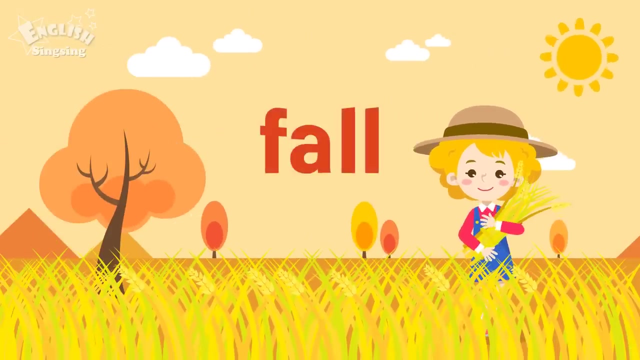 Vacation, Vacation, Vacation. I love summer vacation, beach, beach. In summer we go to the beach. summer, summer It is summer. fall: cool, cool, Fall is cool leaves, leaves- The leaves are falling. harvest harvest- Fall is the season of harvest. fall, fall It is fall. 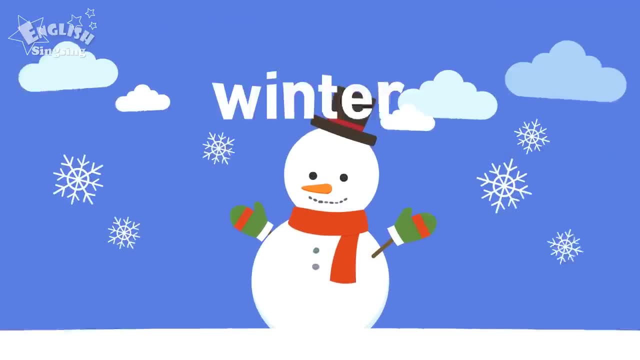 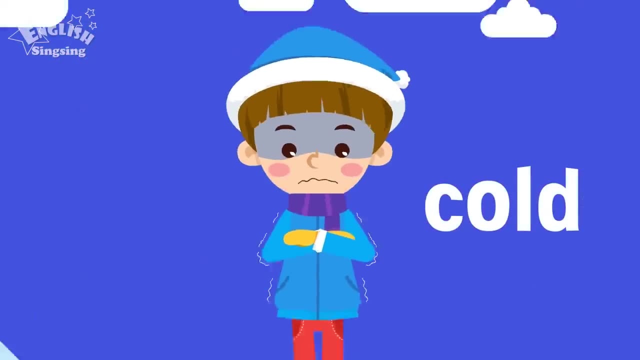 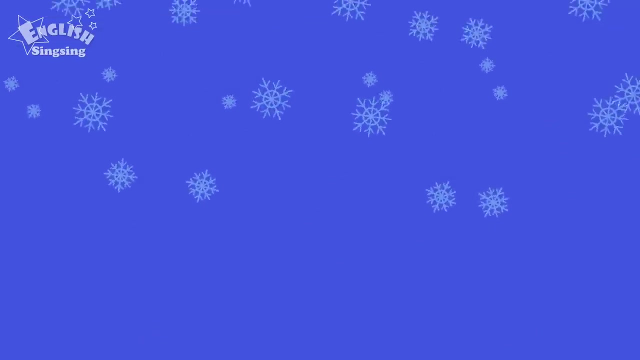 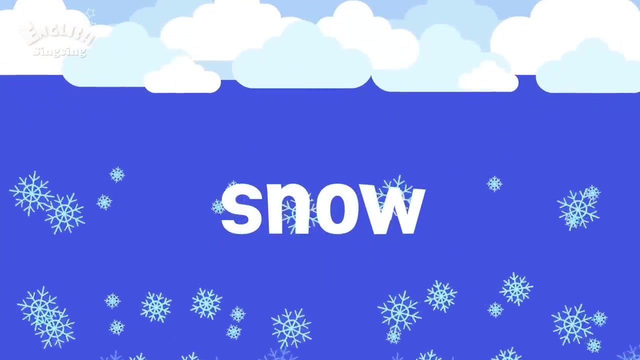 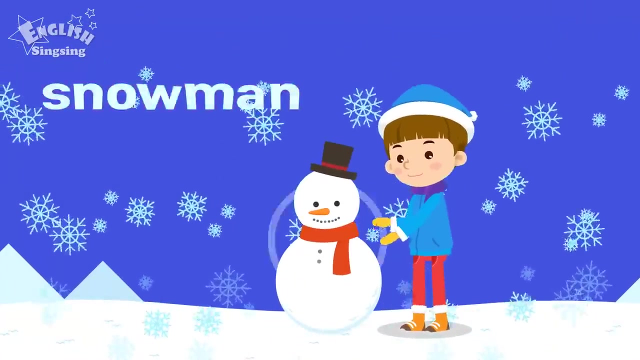 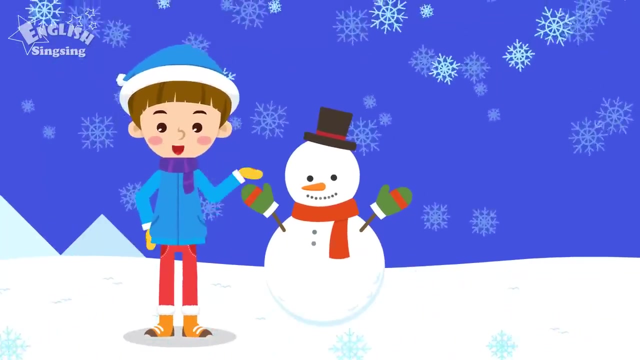 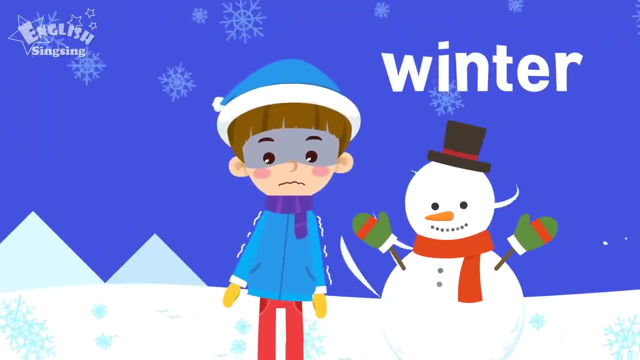 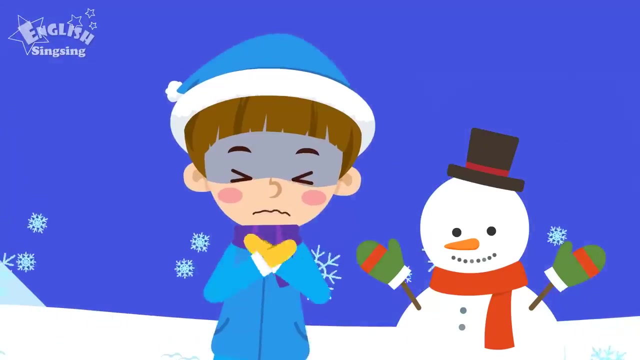 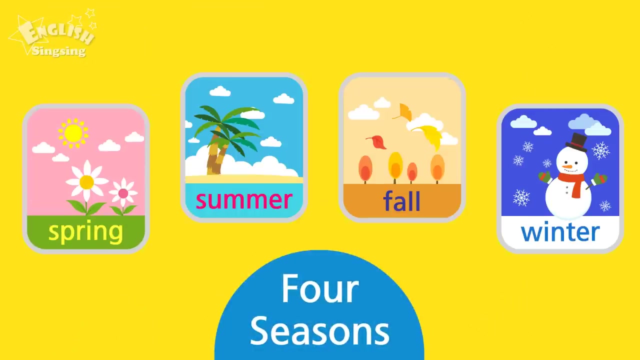 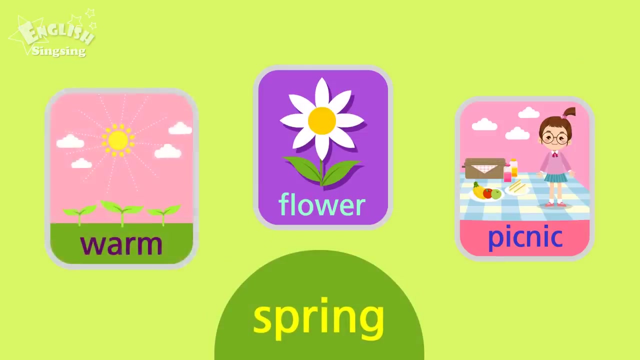 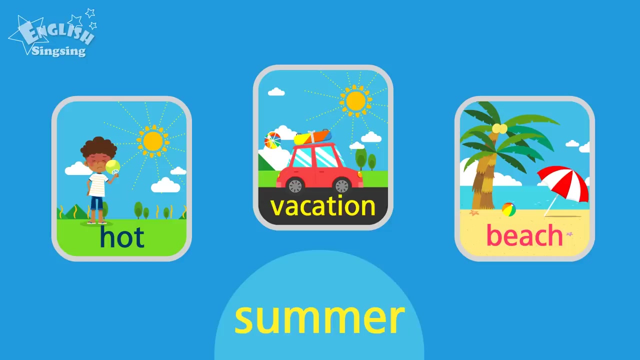 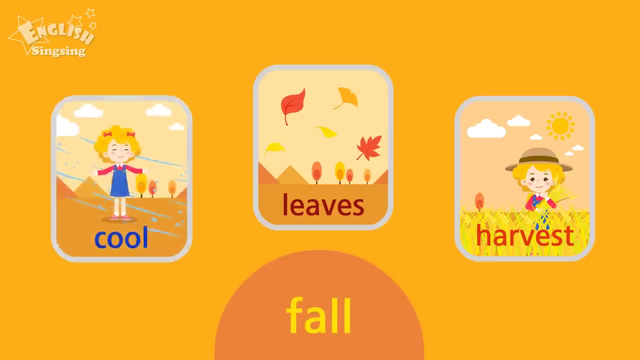 fall winter, cold, cold, Winter is cold, snow, snow. It snows a lot in winter. snowman, snowman, snowman, snowman. We are making a snowman, winter, winter, It is winter. review four seasons: spring, warm flower picnic, summer, hot vacation, beach, three months.